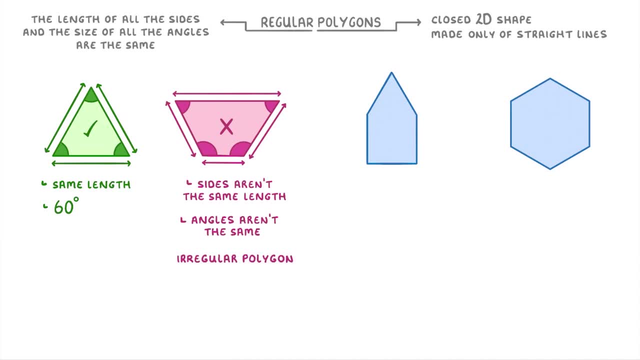 Or because it has four sides, which makes it a quadrilateral. to be more specific, we could call it an irregular quadrilateral. Then this third shape, which is a pentagon, because it has five sides, also wouldn't count as a regular polygon because, although its sides are all the same length, its angles 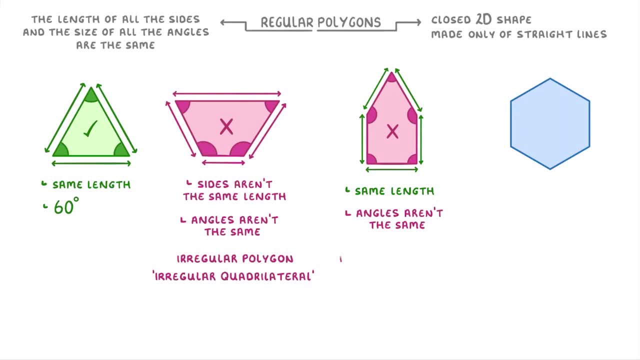 aren't all the same size, And so it would count as an irregular polygon, Or an irregular pentagon to be more precise. And lastly, the shape on the right would count as a regular polygon, because its six sides are all the same length and its six angles are all the same size. 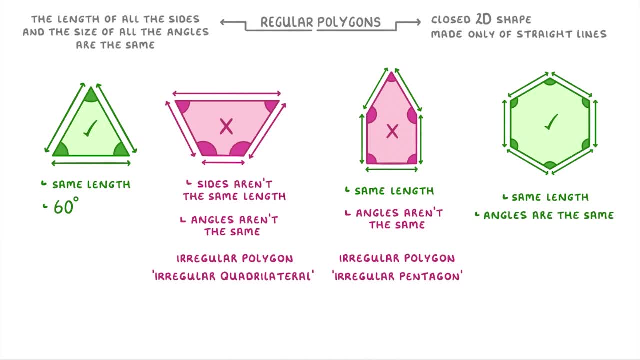 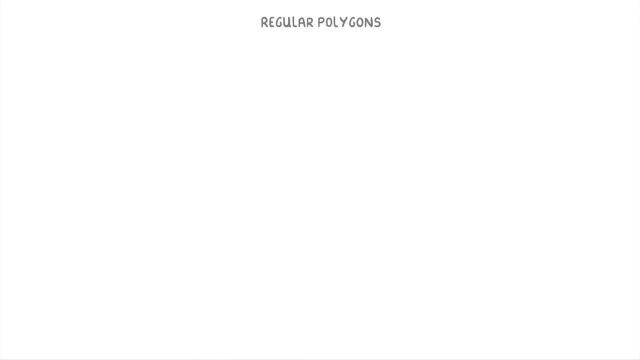 And because its six sides make it a hexagon as well as a regular polygon, we could call it a regular hexagon. What we're going to do now is run through all the main regular polygons, Starting from an equilateral triangle, which is the smallest, and then adding one side. 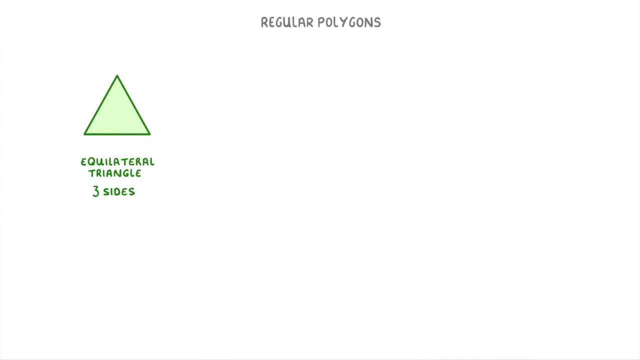 each time. So next we'd have a square which is a regular quadrilateral, then a regular pentagon, then a regular hexagon, a regular heptagon with seven sides, a regular octagon, a regular nonagon with nine sides and finally a regular decagon which has four sides. 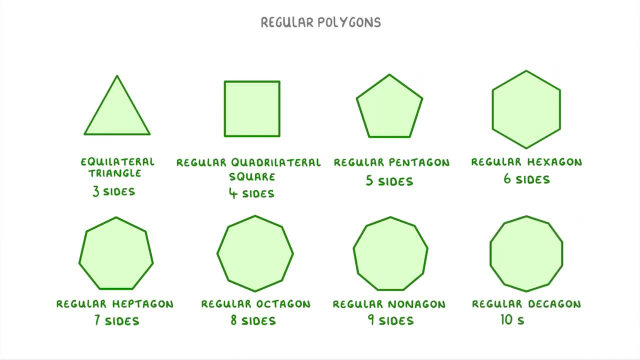 And finally, a regular hexagon, which is a hexagon, and a regular octagon, and a regular hexagon which has ten sides. Now, one of the nice things about regular polygons is that they all have the same number of lines of symmetry as they have sides. 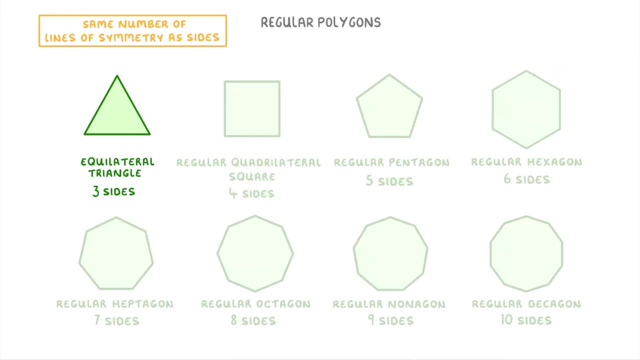 For example, a regular triangle which has three sides will also have three lines of symmetry, while a regular hexagon which has six sides will have six lines of symmetry, And the same rule goes for all the others. They also have the same order of rotational symmetry, as they have number of sides. 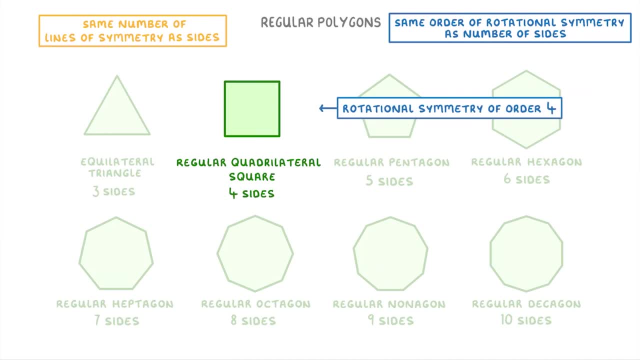 So a square which has four sides will have a rotational symmetry of order four, which just means that with one complete rotation of 360 degrees, there are four positions where the square will look the same, For example, if we mark this top side so you can follow it round as it rotates the square. 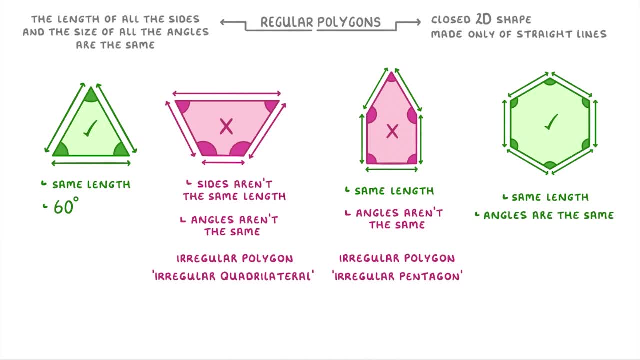 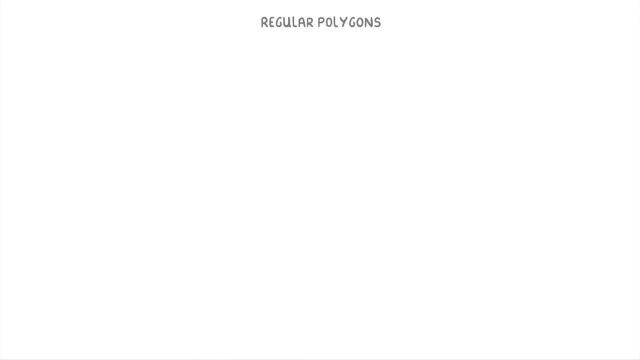 And because its 6 sides make it a hexagon as well as a regular polygon, we could call it a regular hexagon. What we're going to do now is run through all the main regular polygons, Starting from an equilateral triangle, which is the smallest, and then adding one side. 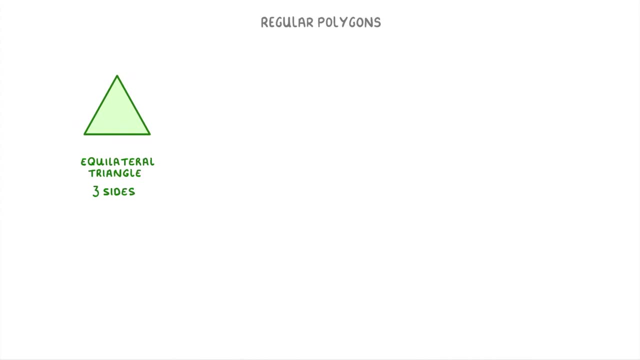 each time. So next we'd have a square which is a regular quadrilateral, then a regular pentagon, then a regular hexagon, a regular heptagon with 7 sides, a regular octagon, a regular nonagon with 9 sides and finally a regular decagon which has 7 sides. 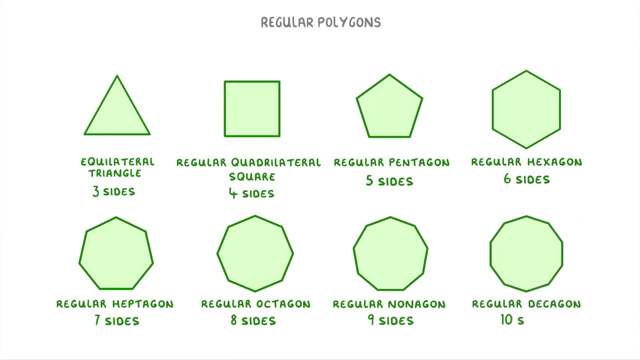 And finally, a regular hexagon, which is a regular hexagon, and then a regular octagon, which has 10 sides. Now, one of the nice things about regular polygons is that they all have the same number of lines of symmetry as they have sides. 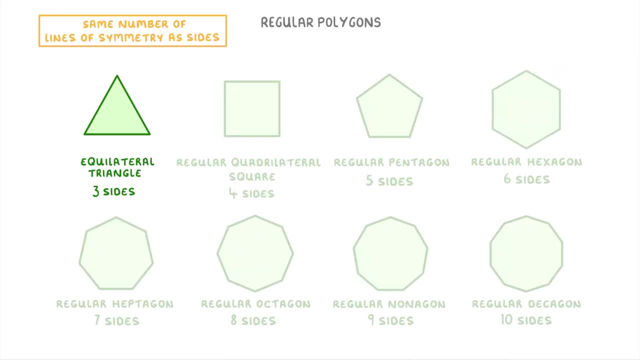 For example, a regular triangle which has 3 sides will also have 3 lines of symmetry, While a regular hexagon which has 6 sides will have 6 lines of symmetry, And the same rule goes for all the others. 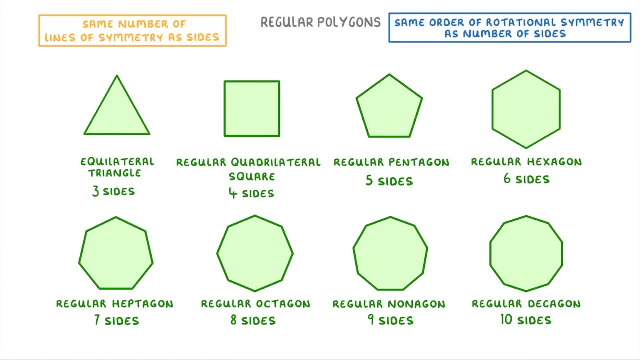 They also have the same order of rotational symmetry as they have number of sides. So a square which has 4 sides will have a rotational symmetry of order 4.. Which just means that with one complete rotation of 360 degrees there are 4 positions where 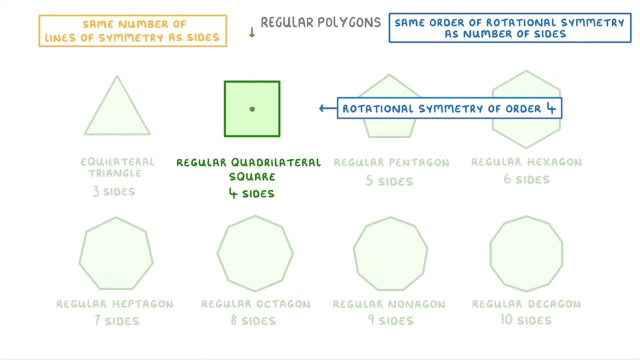 the square will look the same. For example, if we mark this top side so you can follow it round as it rotates, the square will look the same here, here, here and here. And if we mark this top side so you can follow it round as it rotates, the square will look. 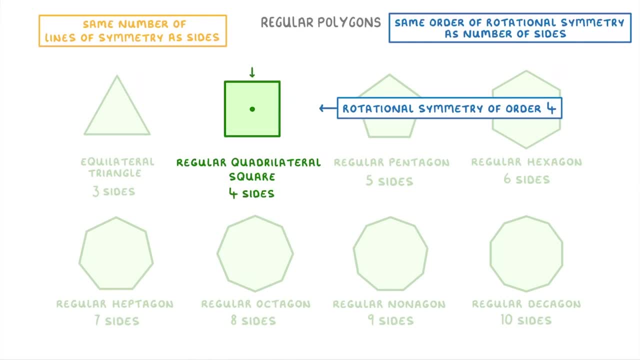 the same here, here, here and here. And if we mark this top side so you can follow it round as it rotates, the square will look. the same here, here and here. And if we mark this top side so you can follow it round as it rotates, the square will look. 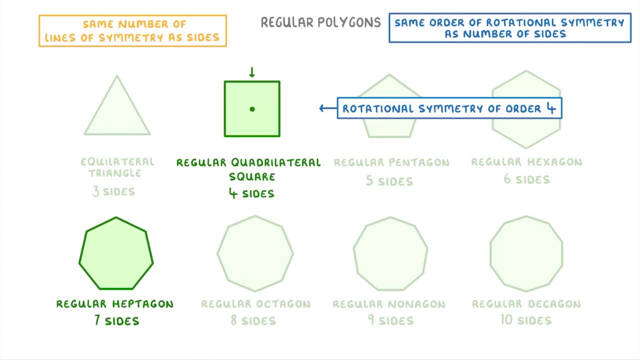 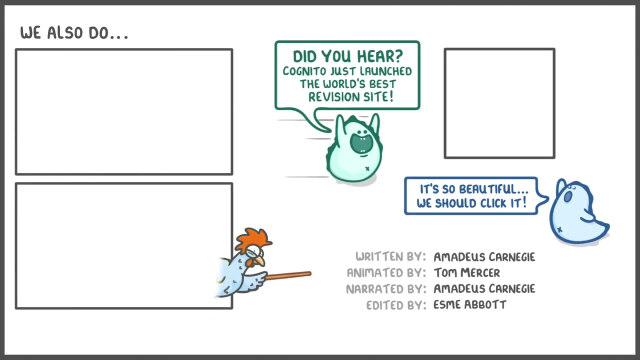 the same here, here and here. And likewise, a heptagon with 7 sides will have a rotational symmetry of order 7. And the same rule applies to all the others. Anyway, that's everything for this video, so if you found it useful, then please do. 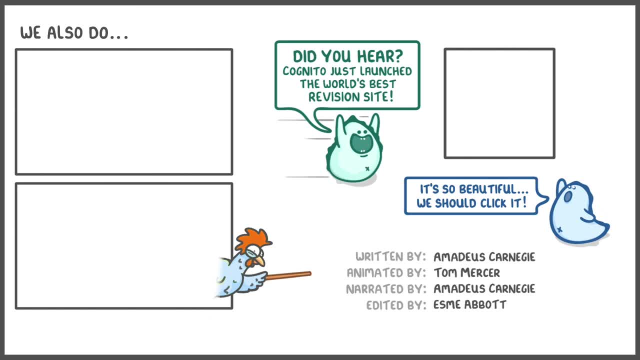 give us a like and subscribe, as it really helps us grow, or tell your friends about us, and we'll see you again next time. Bye, Bye, Bye, Bye.